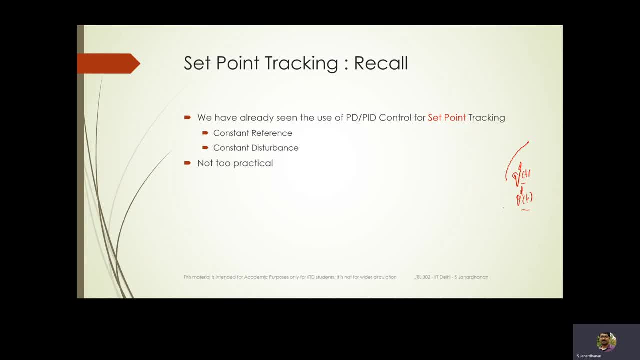 And I have to generate a control such that this, my actual theta M or Q follows this reference. Okay. And similarly, the disturbance that we have assumed the disturbance to be the summation of the gravity term and the cross coupling terms in the Coriolis matrix Q, Q dot, the cross coupling in the Coriolis force, that is being considered as a disturbance. 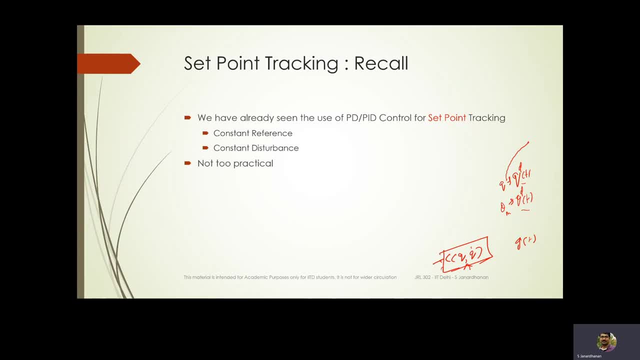 And since Q is a time varying quantity, you can expect this, you can't expect this to again be constant. Okay. Similarly through the gravity. The two. 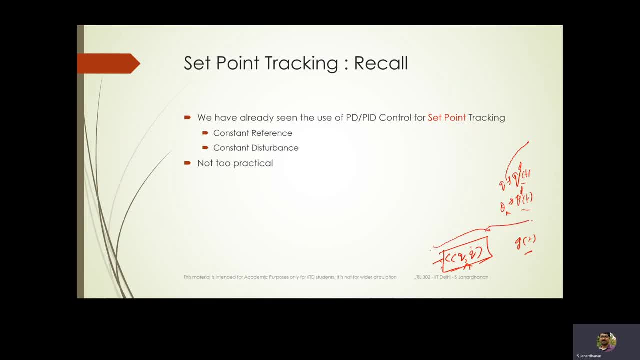 Totally ignoring the time varying nature of this is going to be detrimental. So you need to have a conceptual takes this factor into account, at least to some extent. That is, you need to have a control that takes into account that the, this is always supposedly a force passat, that is, you need to have a control that takes into account that these 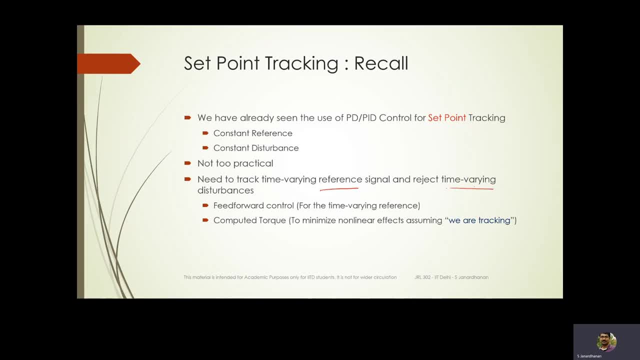 reference signal can be time varying and the disturbances can be time varying okay so you can so in this session in this lecture we'll be talking about two concepts 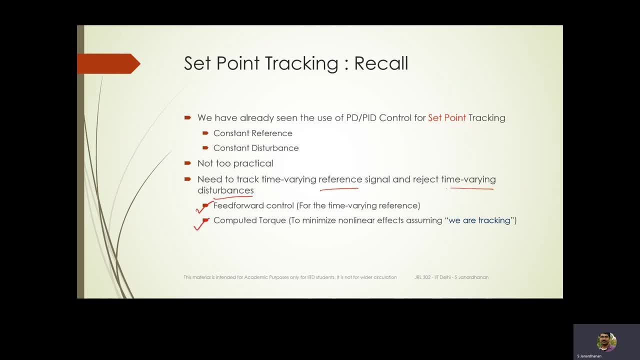 of our control that is one is the feed forward control and one is a computer control 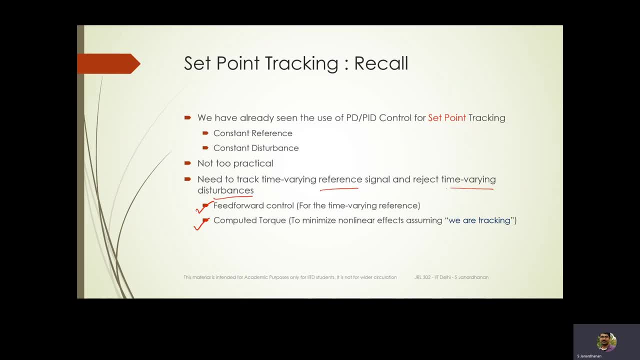 so in the feed forward control part you will be handling the need you will be compensating you will design a control that compensates for the time varying 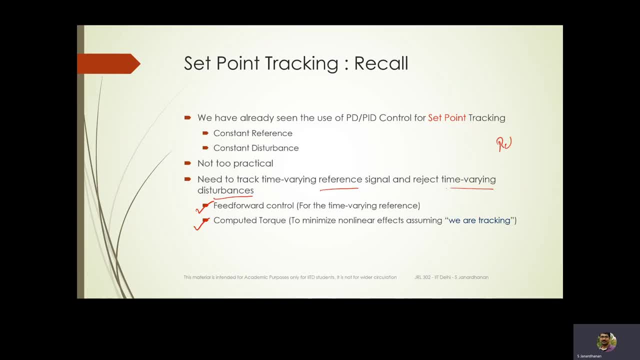 nature of a reference assuming that the reference is known a priori so if you have theta d as your reference theta d is known beforehand this function theta d is known beforehand 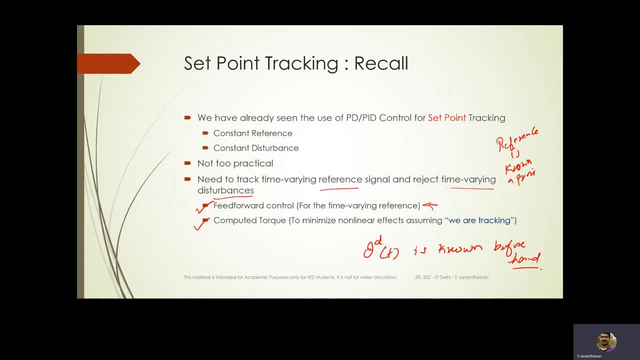 okay and in that case you can generate a control signal that that tries to compensate for this time varying nature of the reference and the other 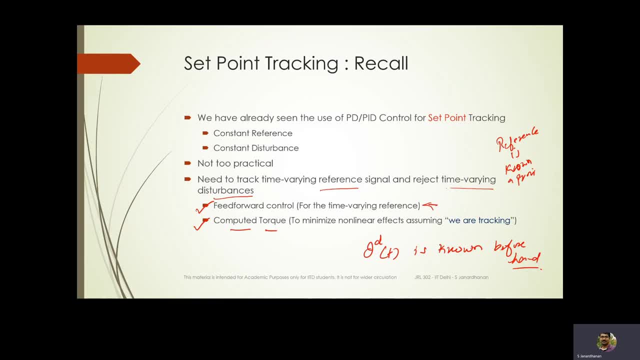 method of control is a computer control which tries to minimize the non-linear effect assuming that you are tracking this reference signal you are already tracking this reference signal and what is the extra control that is needed to 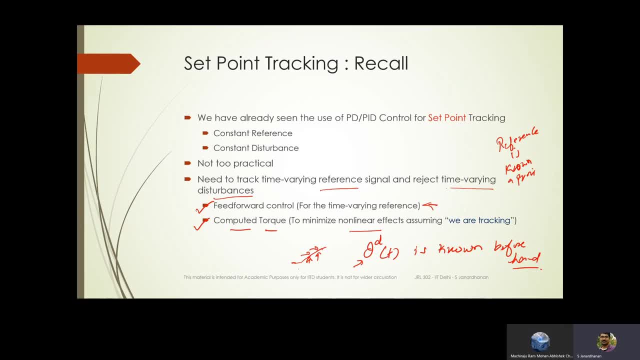 a non-linear effort so that you keep on tracking the control you maintain the tracking okay so that is the computer control part of it we will go into both of these concepts one by one 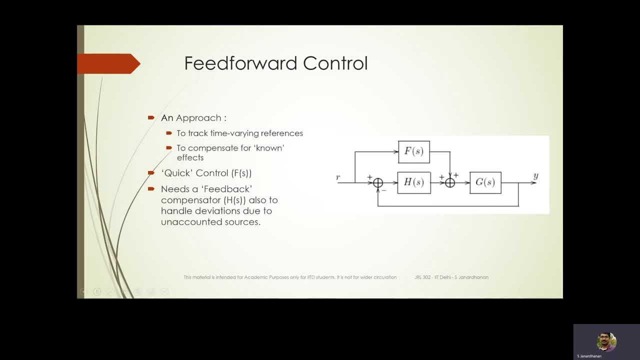 so first we look at the feed forward control so here what you had is what we had uh handled uh in in the last lecture was that this h of s was a pd or a prd controller and this was 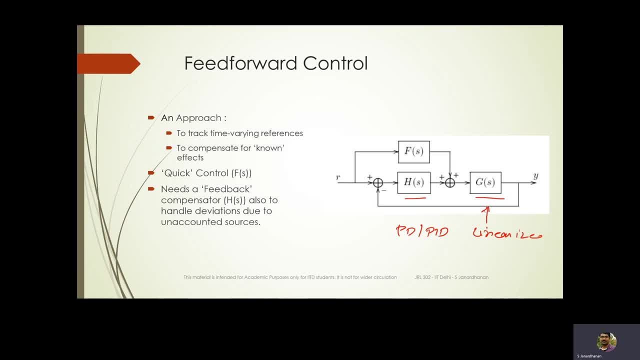 your linearized uh manipulator dynamics so linearized joint dynamics which was of k by something into j a square plus bs something of this sort okay and this r was assumed to be a constant signal 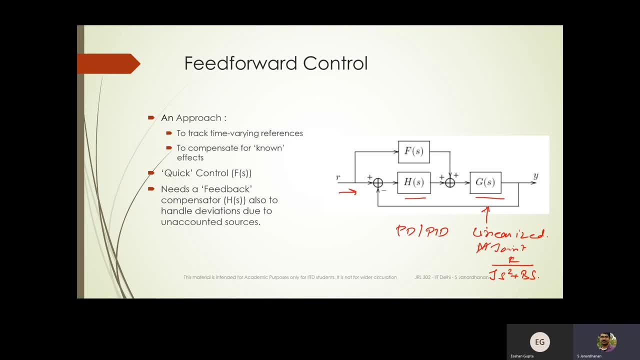 okay now in this lecture we will start with addition of this f of s which is the feed forward control part notice that f of s this signal depends only on what is our office it doesn't operate on this error at all okay and this uh this feed forward signal is an approach that can be used to track time varying references and since it doesn't operate 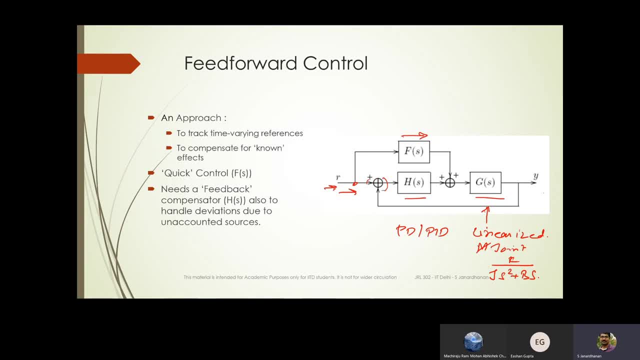 on the feedback it doesn't require the measurement signal at all it doesn't require the measurement of y because let us say let us take a qualitative view on this see when will when will this signal h of the output of h of s when will it react to any deviation so what should happen is there should be some error and because of that that error propagates in from g of s it will appear in the 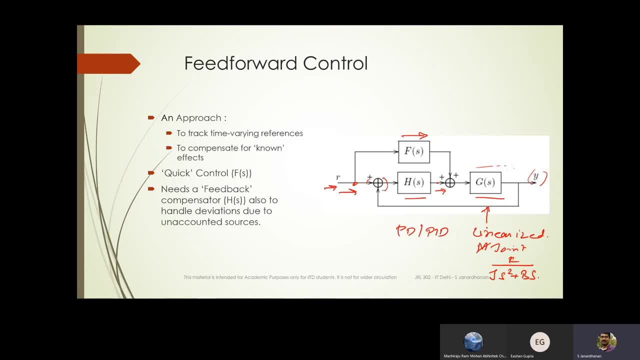 it will appear in the output this output should be compared with the yeah this should output should be compared with your this output should be compared with your reference signal and only when that error is realized you see a change in a corrective action in hfs so it the feed for feedback path takes into account any error that is happening 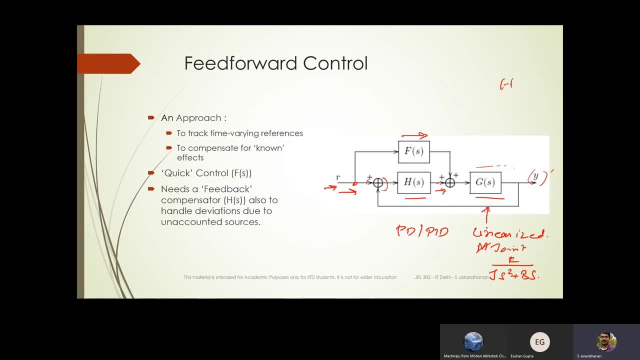 however it is slower so feedback is a little slower but it is more reliable 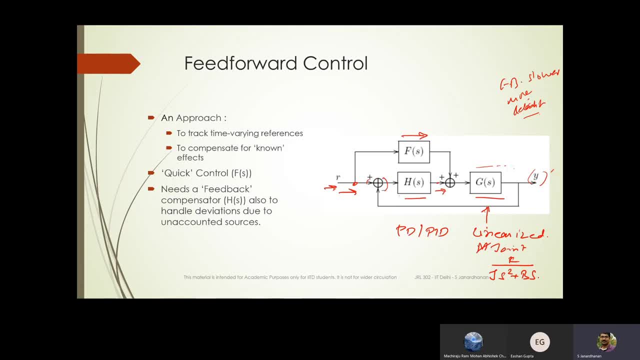 okay the feed forward path is quick because it doesn't it doesn't require an intervention from the output it doesn't require a measurement of the output the feed forward control is a quick control okay however since it doesn't take into account any error the the compensation for the error for the compensation of error you need the feedback path also so both h of s and f 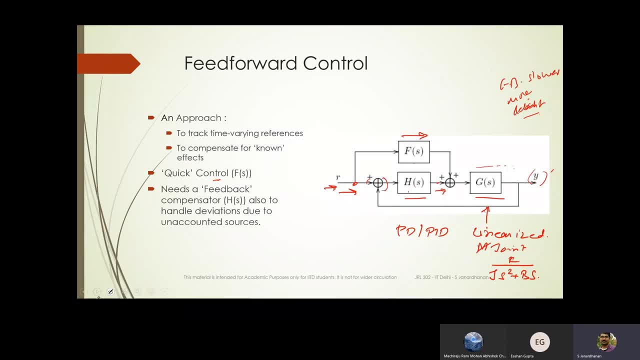 of s is needed okay now let's see what happens okay what happens to y and how is it dependent on r when a forward control is added to it so this signal e1 at the first summing point is just r minus y e2 is a summation of h times even plus f times r okay and y is g times e2 so if you try to solve this uh for what what is what was y by r you get this expression okay you get this expression you get g times h into f plus 1 plus gh okay now what would happen if you if you were to choose f of s as 1 by g of s so if you choose f of s as 1 by g of s your y by r term your y by r will turn out to be g h plus g into 1 by g divided by 1 plus g h this turns out to be 1. okay so which would mean that you have perfect tracking 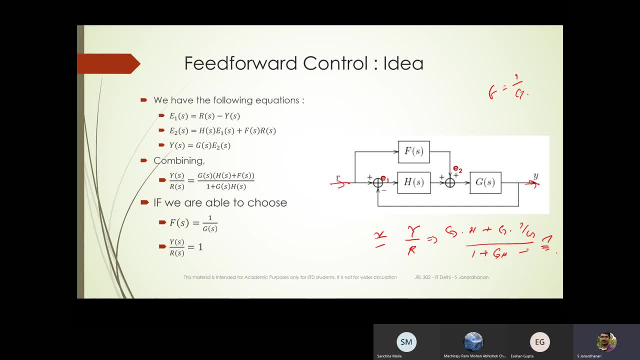 due to the application of your feedforward control okay so even if your r office of course if even if you know if r of s changes this f into f of s into r of s is going to be another signal that 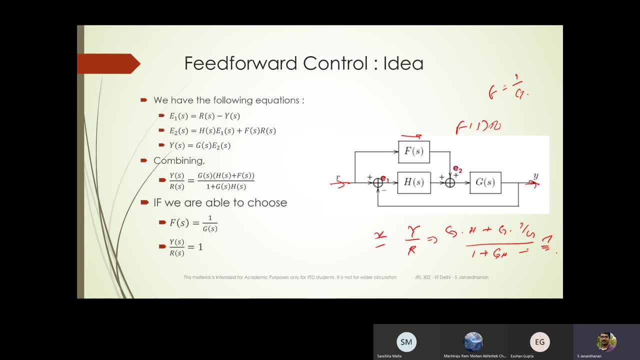 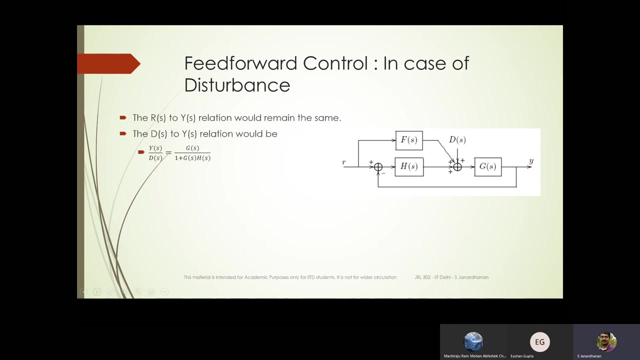 compensates for this trick shadow android why it's called shadow android the second thing that it's going to do is it's going to it's gonna of this szyb the output 겁니다 of says we have that signal sets for the change in R of S that is going to add a corrective signal and try to maintain Y to be equal to R. Let us see what if there is any problem in that. Now let us say that if you instead of but for now we have only accounted for a change in the control R and we have not yet added the disturbance component of it. So let us add another disturbance component D of S that is affecting the system. So in our manipulator case this D of S is the cross coupling terms. So this is the cross coupling term that comes in the manipulator. So in our manipulator case this D of S is the cross coupling term that comes in the manipulator. 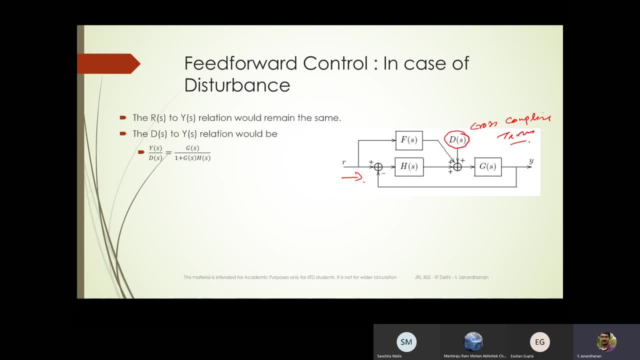 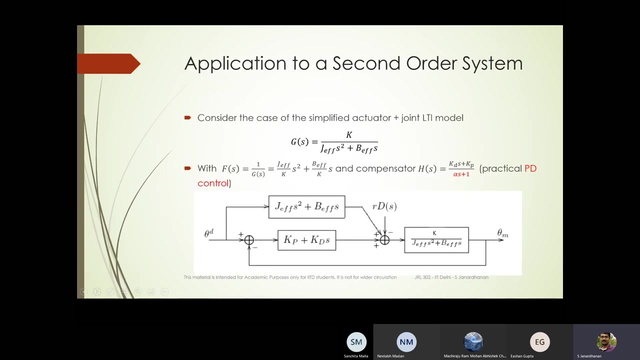 So in our manipulator case this D of S is the cross coupling term that comes in the représence of this feed forward path. Now let us see that how D of S will affect Y in presence of this feed forward path. You would see that this feed forward path if you look into if you just set R equal to zero and try to see what is Y by D you will get this transfer function g by 1 plus gh. And if you add that to your already existing signal you get a which is r minus y to be a function that is dependent on your disturbance alone okay so your steady state error is only due to disturbance this is very similar to what was happening in case of your pd control and even in pid controller so if the disturbance were constant and you use a pid control with constant disturbance okay you will get the steady state error to be equal to zero okay so if there was a constant disturbance the steady state error is zero but we have to take into account that the disturbance need not be constant okay so maybe some other extra component is to be needed to minimize the effect of the disturbance also but before that let us look into the how we can apply the feed forward control in case of the robotic manipulator control control of the manipulator joint so the simplest case was P we 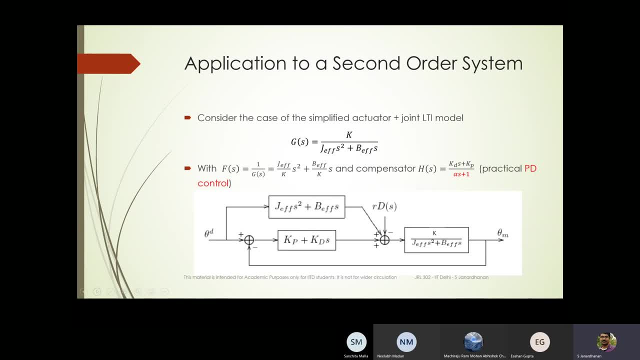 had the joint model and the actuator model combined together to get a second-order equation K by J square plus B 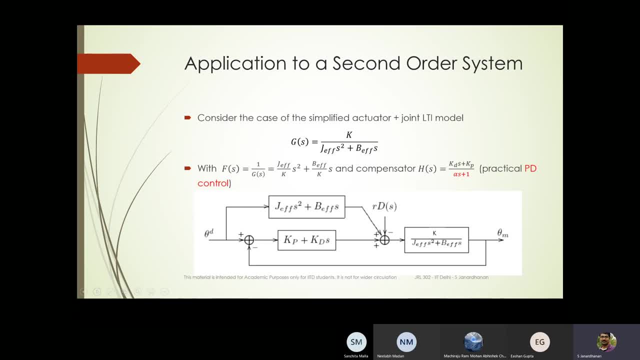 bfs and what what we had learned from the feed forward control was that we have to choose the feed forward control to be one by g of s so if you choose feed forward control to 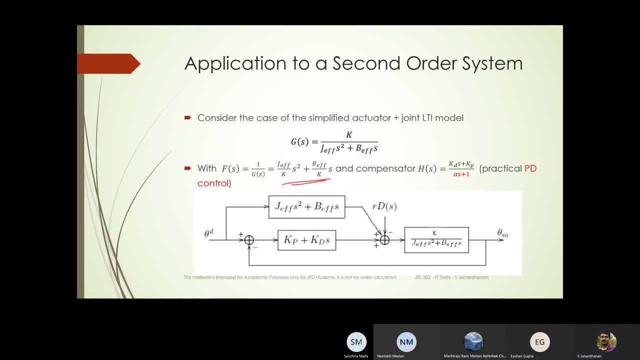 be one by g of s you get an expression like this okay now that would mean that if you have theta d okay then uh this signal what what comes at this point okay let us say if 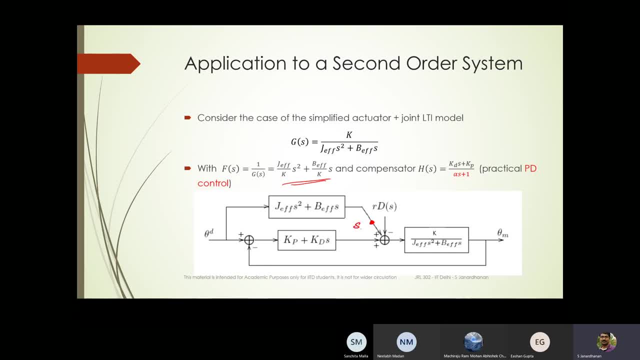 this is say uh you say this is s1 okay so s1 of t would be equal to j effective by k times the second derivative of theta double dot plus b 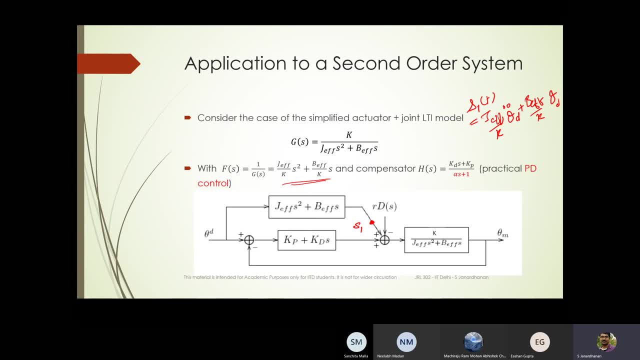 effective by K into the first derivative of theta double dot. Okay. Now the question that I want that I'm posing is that isn't this anticipatory? Okay. So what we had said is that so the question that I had posed now is that whether this would be because your control now your control that you have here. Okay. Is something of the form some constant into second derivative of your desired reference signal plus something into the first derivative of your desired reference signal. Okay. However, in the last class, I had told that when you 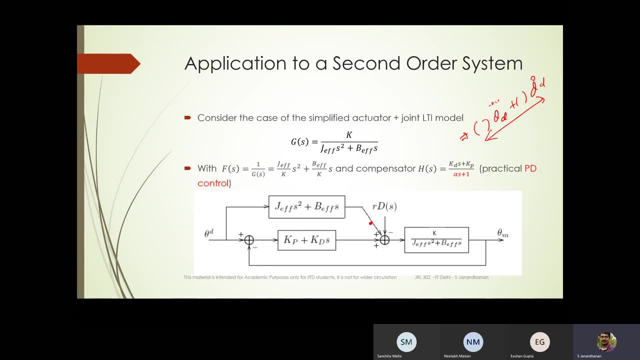 have this derivative, say the first or second derivatives, then the control is anticipatory 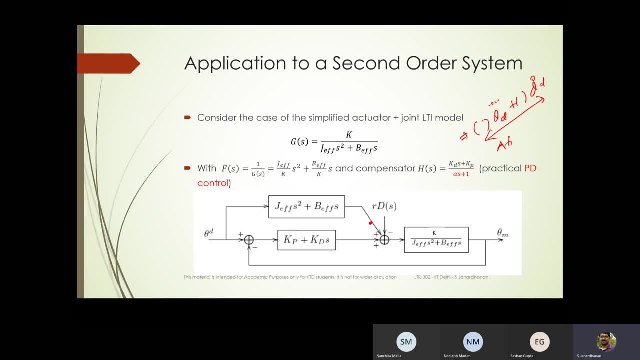 and anticipatory control is not really implementable. Okay. So the question is, here is that is this actually a practical solution when you so because I had just told it anticipatory control will not work, then I'm proposing a control that is completely 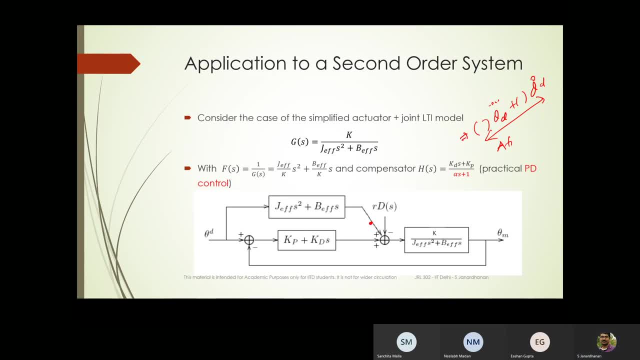 anticipatory. So what is your view on that? Yeah, so the, the change here is that anticipatory control is not 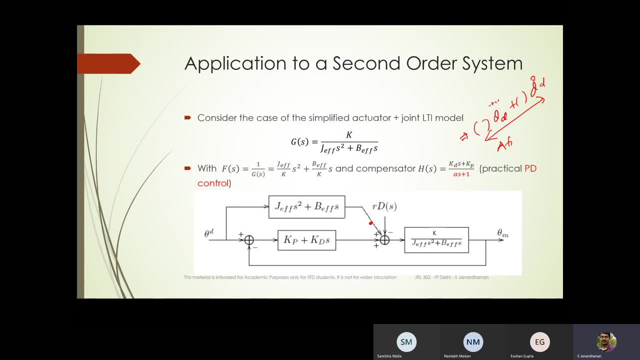 feasible in case the derivatives taken are for measurement. So the point is that derivatives or time derivatives of measured signals is something that you can't guarantee because I don't know how the measured signal is going to evolve in the future. That is something that I can't comment about. So this is not possible. However, time derivatives are possible. So that makes sense. 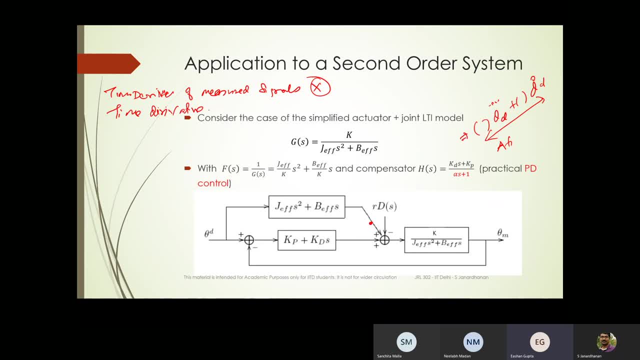 Presenter 2 Sir, what do you mean by measured signals like signals that we can measure in some means. 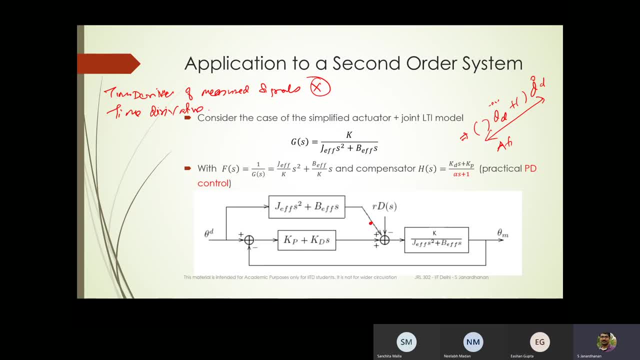 Presenter 3 So in the sense that in the sense that let us say that you want your let us say you want your some joint to follow sinusoidal trajectory. 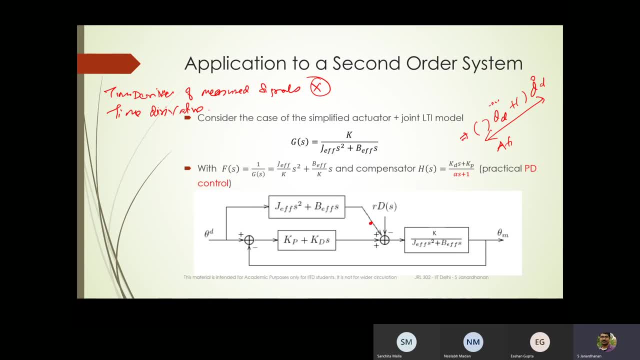 Okay, so that is your aim. So I know to, I know to take the time derivative of a sine wave. I say that that will be Omega Cos Omega k there is no problem with that. So it will be Omega Cos Omega k. So the derivative of sine wave means the time derivative of a wave. So this is the derivative of time derivative. The derivative of time derivative of sine wave. 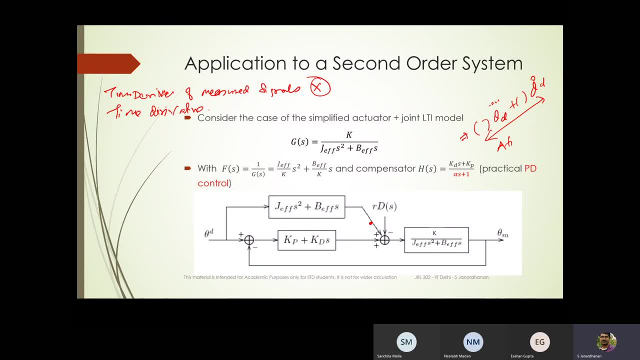 however I don't know if the joint is going to follow that trajectory maybe it is possible that I have got a wrong model okay so if I apply this signal I don't know if the if the joint is it will exactly follow that trajectory the only way that I can even verify it is to actually measure using some what you call some sensor I have to measure the actual joint angle okay so I will be able to measure the joint angle now I will have history of what was the joint angle in the past but I have no idea what will be the joint angle in the future 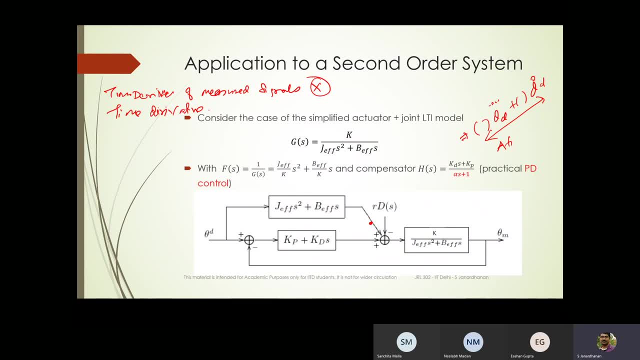 okay is that clear yes sir yeah so so if for since I don't know what will be the future of a measured signal of our of a signal 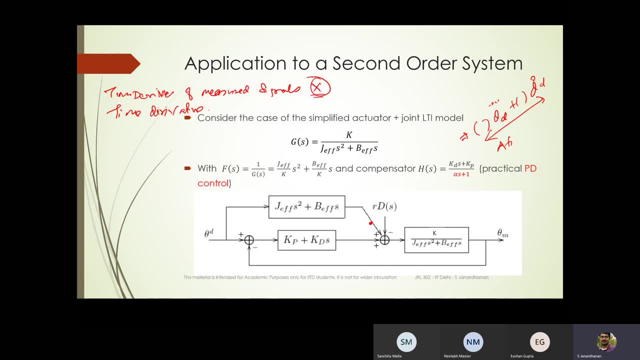 that I have to measure I cannot rely on having d by dt of any measured signal that being an integral part of my control even if it looks like that the controller structure should be in a manner that I don't I would not need to use the time derivative of any measured signal okay however it is for reference signal it is okay because reference signal is something that I desire to have so if I say that I want it to follow a step step signal then I can compute the time derivative of steps like I do in some mathematics course on mathematics I will compute 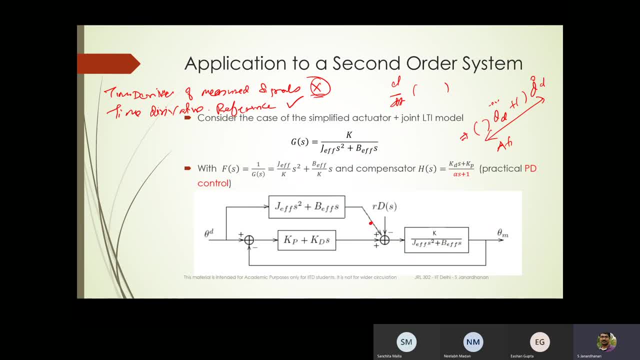 the time derivative of a signal of any mathematical signal and apply and say that this is my d by dt of 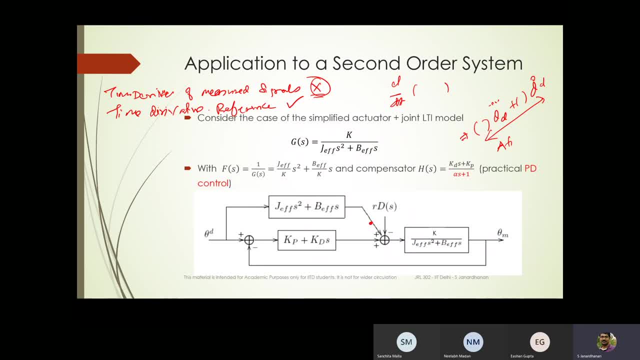 my reference that is well and good so this thing is okay f of s can be in this manner however if I choose a if I 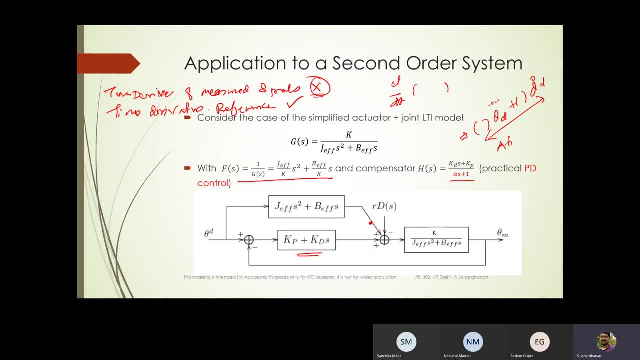 choose a pd controller for my feedback compensator the pd controller is not of the structure the pd controller has this denominator to make make it a practical pd controller okay so that's the way 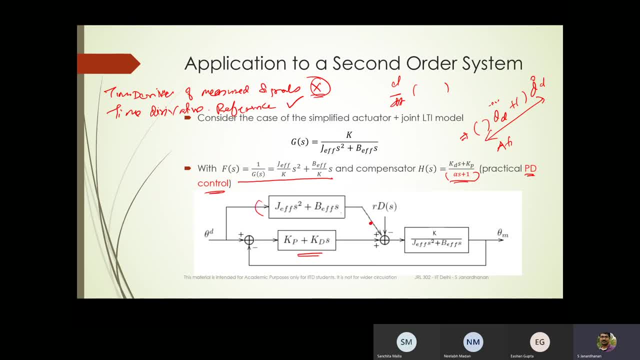 that's that's the structural difference that would have that you would have between the feedback feed forward control and the feedback control okay now this is the control that you are applying into 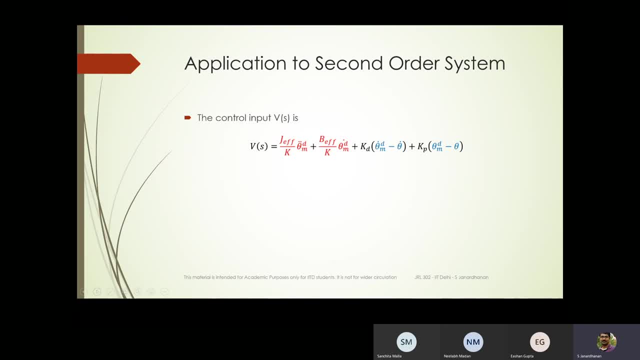 your system so if you combine the feedback path and the feed forward path so this is the feed forward control this is the feedback control that you have okay and if you add both of them together if you add both of them together you get a controller structure like this 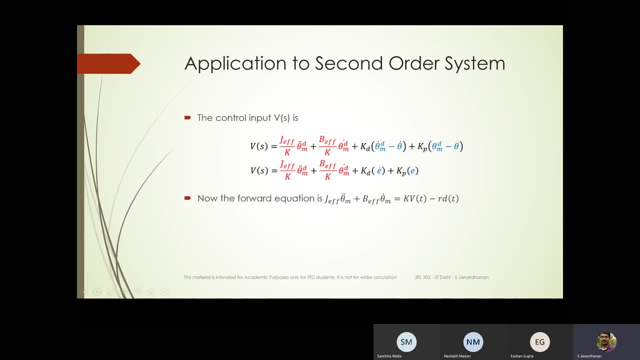 means the control structure like this and now if you see 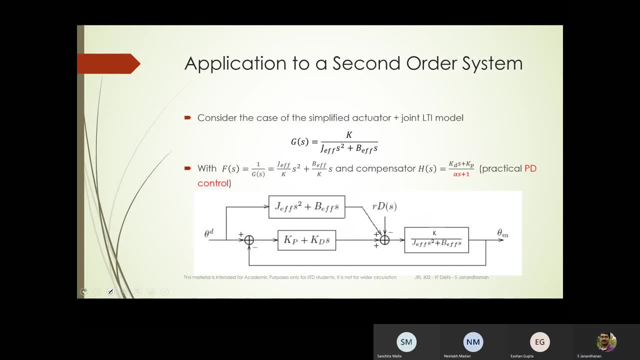 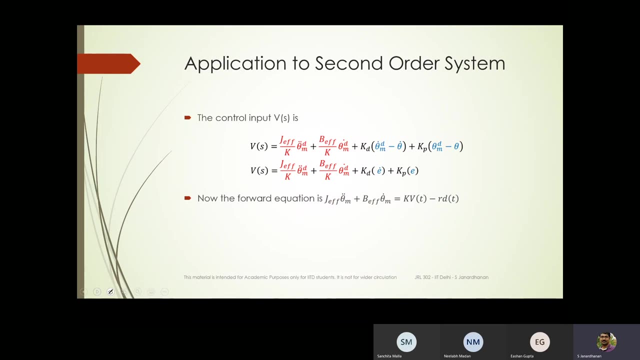 the forward equation if you go back okay this was whatever was here okay at the relationship with what what what was a signal here and what was a signal here is given as uh by this equation so j effective times theta m double dot plus b effective theta m will be this signal that is the input signal and 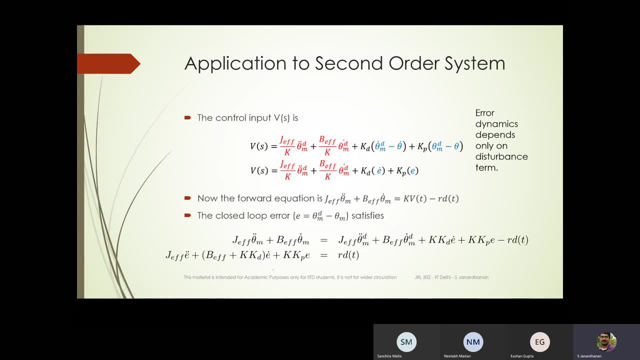 if you write it out and if you say error is theta m d minus theta m you get you find that the dynamics of the error is 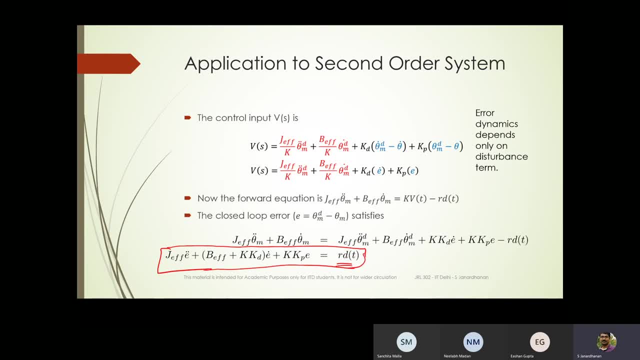 dependent on what was the disturbance alone this was again this is again similar to the case that we had in the in the case of the pid controller 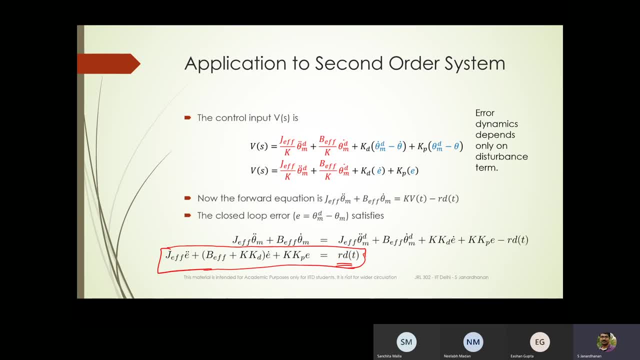 and again this will become this will be trivial in the case when you have when if you apply like if you apply prd controller with d being constant there is no problem even now okay however what has 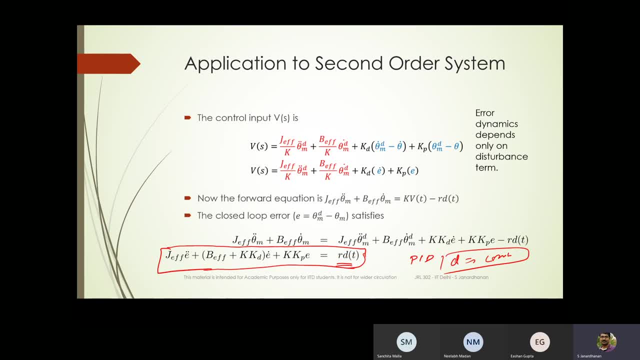 been uh the first problem that has been solved is that now the reference need not be i can track any reference that changes with time but if the disturbance changes with time then i'll have 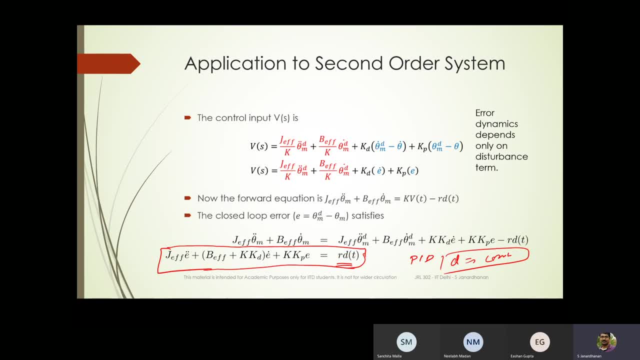 an error that is proportional to the magnitude of the disturbance or presented on theyard so if theまぁ sometimes the path is or yeah then it will be proportional to the magnitude of disturbance that will that you will have here uh and as long as j effective 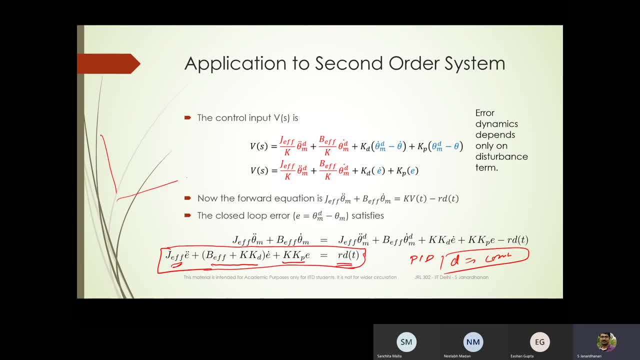 this expression and this expression all of them are positive the dynamic is stable so you would if you see the error the error may start from some value if you say e of t versus t error will start from some value and it will go into some band this band 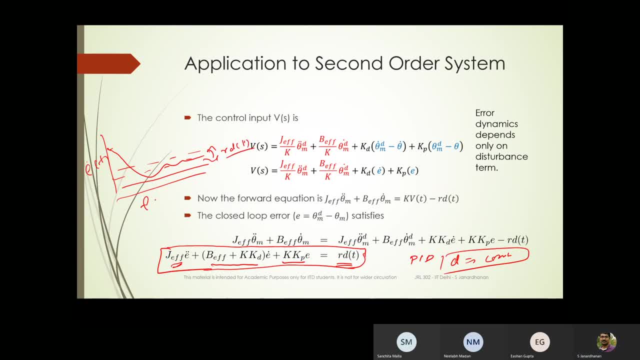 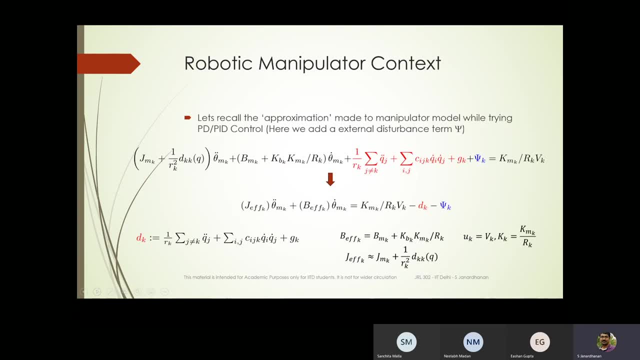 on the magnitude of RD of T. Okay. However, no, no, let's go back to what we had considered as D of T in the earlier case. So this was, it comes to the same thing. So you had come, we had considered that this was this term, this entire term was J effective that is accounted for this entire term was B effective that also we had accounted for. And initially we had taken whatever was in red as D of T. Okay. And this, these are effects that we had, uh, that were part of the dynamics of your manipulator model itself of joint model itself that were actually ignored and clubbed as a disturbance. Okay. Now let us add one more term. This are . external factors, okay, maybe there is some something, some say play in the gear, there may be there is some measurement error or not measurement error, there is some external factor, some disturbance, some extra disturbance that is affecting the system that is not actually accounted for by the model itself. Let us say that is the psi, okay. So, these are external disturbances that are affecting. We do not know how, we have no way to even model how it is affecting the system. So, there is a minor effect of this, okay, that affects how the manipulator is moving, how the manipulator joint is moving, but I do not have any model for it. Only have is 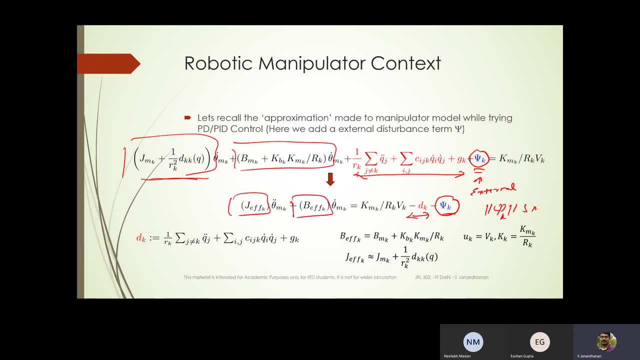 that it is of a small magnitude, okay, there is a small magnitude disturbance that is affecting which is external. 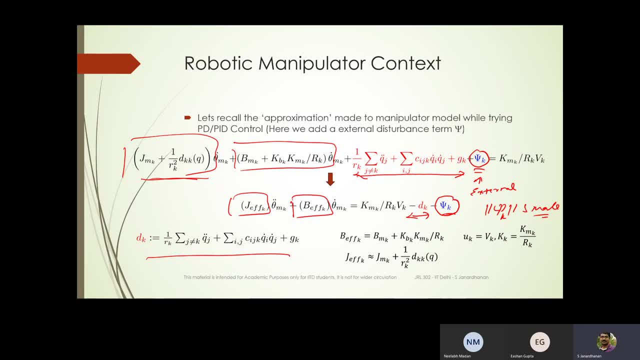 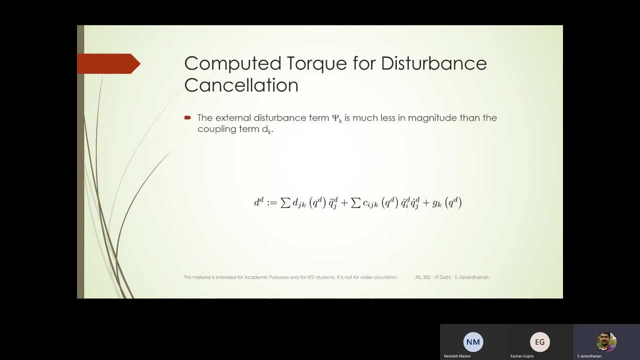 Okay, and this d of k, as we said, is equivalent to what the cross coupling effects and the gravity term that is added. Okay. Now, what we are doing is that we have this, we have this term as psi k, which is the external disturbance, which is much less magnitude than the 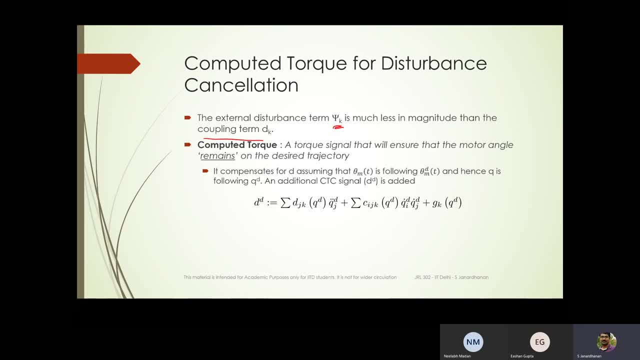 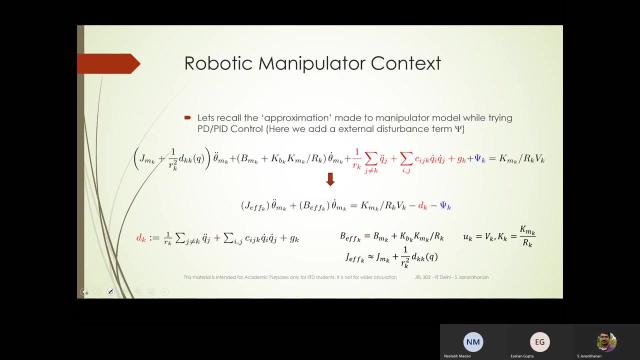 cross coupling term dk. And we use the computer torque, which would be this dk, assuming that q is equal to q desired, okay. Assuming that the manipulator is following the trajectory, there would have been some value for this error. That means this cross coupling term dk. And we use the computer torque, which would be this dk, assuming that q is equal to q desired, okay. Assuming that q desired, okay. Assuming that q desired, okay. 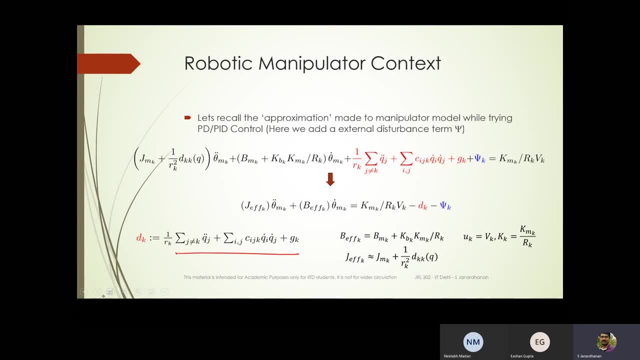 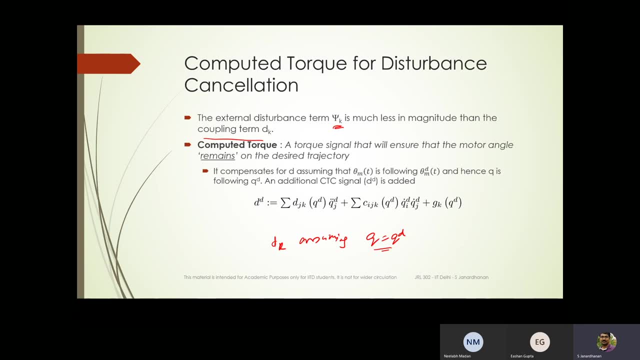 Now, what we can do is this, we can take the number of these cross coupling terms, okay, and that is taken out, that is computed as your d d. And that is the computer torque signal. It is that signal that will ensure that the motor angle remains on the desired trajectory. 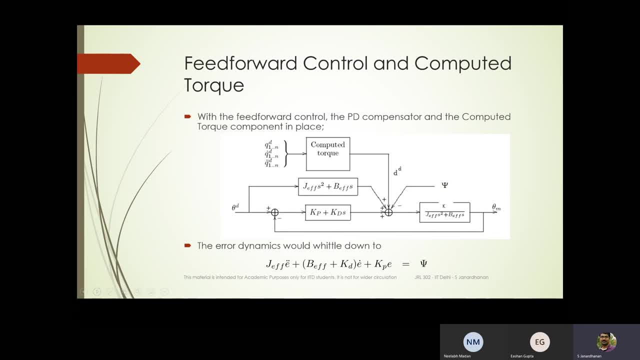 Okay, now if you write it in this manner, so instead of, so you had a disturbance, a term here. Okay. Now that disturbance term need not be taken at all because here you have, you don't have this J effective. You have actually the manipulator. Okay. So in the manipulator dynamics, you had this DK and that is compensated with this DDK. Now if you take both of them together, effectively you end up with an equation in which the right hand side, instead of being dependent on the entire D plus side is now only dependent on side. And as we had taken earlier, this term side is, has a much lesser magnitude. The external disturbance factor has much less magnitude than the cross coupling terms.